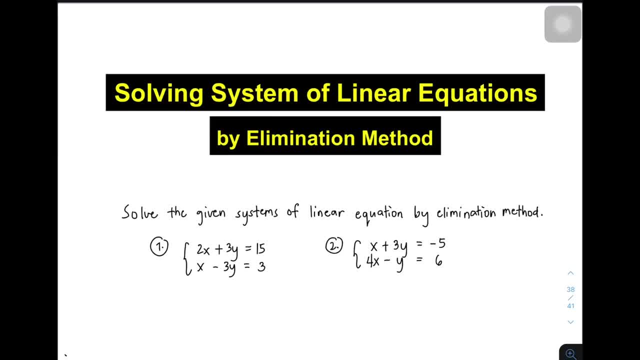 Hi guys, it's me, Teacher Gon. In our today's video, we will talk about solving system of linear equations by elimination method. Last time we are done uploading how to solve system of linear equations by graphical method and substitution method, So the focus of today is on how to use elimination. 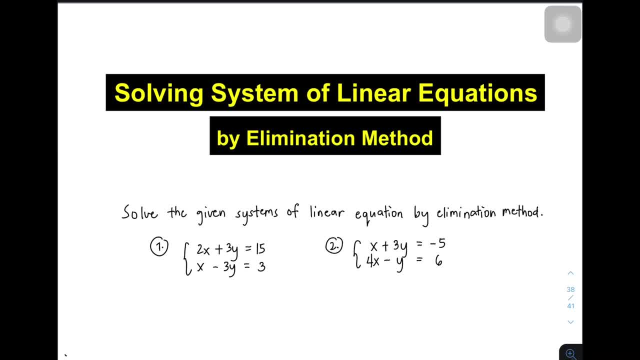 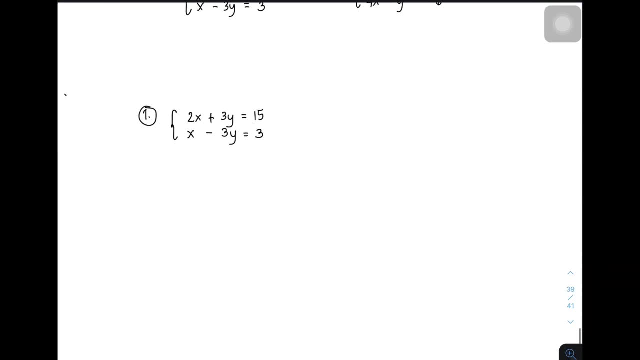 method or addition method to find the solution of the given system of linear equations. So we have here examples number one and two: Solve the given systems of linear equation by elimination method. So without further ado, let's do this topic. So we have example number one. 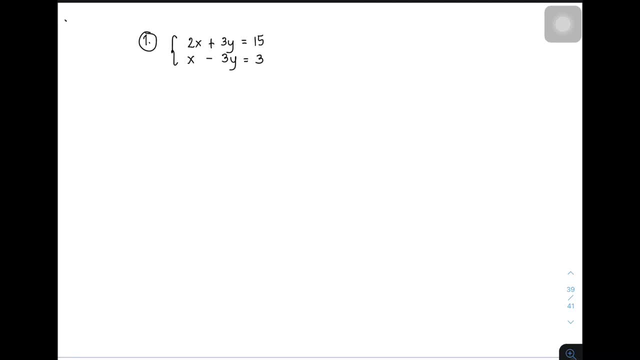 The given system is: 2x plus 3y is equal to 15, and we have x minus 3y is equal to 3.. This is your equation number one. This is your equation number two. Our target here is to eliminate a single variable for us to find the other. 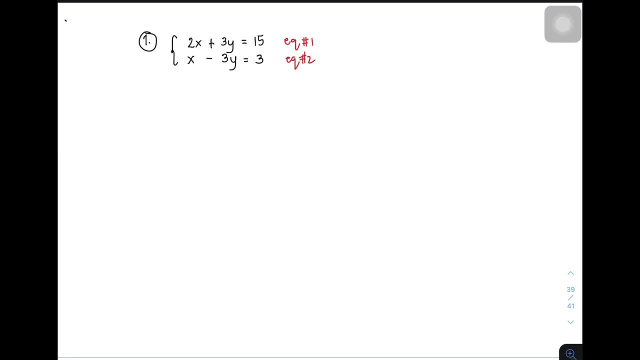 So again, our target is to eliminate one variable so that we can solve the other variable. So how First find a variable with the same coefficient but with different sign? So here in this problem- this is what I said- We have three. 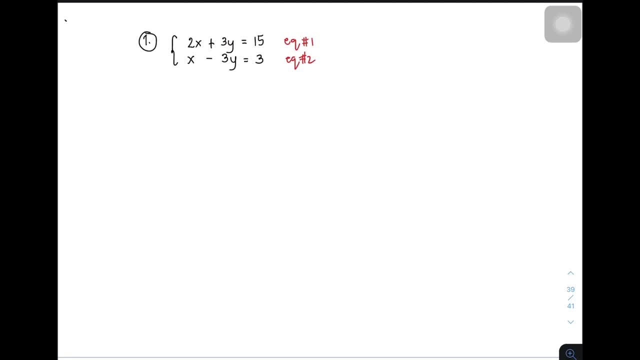 and negative three. This means we can eliminate the variable y. So let's copy this. You have: 2x plus 3y is equal to 15, while the other is x minus 3y is equal to 3.. Another thing that you need to: 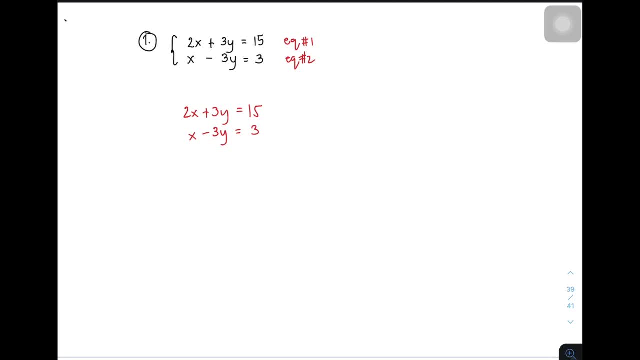 remember is you need to align the terms with like variables or same variables, so you can easily apply the elimination method And then, right after this, add that to sila. Add So here this is equal to zero or we can cancel it out. 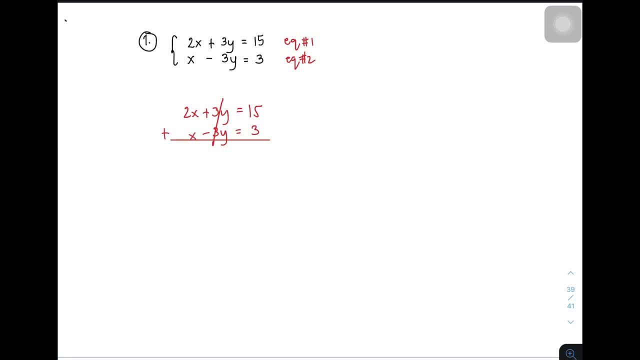 So we can add these two terms: 2x plus x is equal to 3x, Then equal to 15 plus 3.. That will give you 18.. So we can add these two terms: 2x plus x is equal to 3x, Then equal to 15 plus 3.. That will give you 18.. 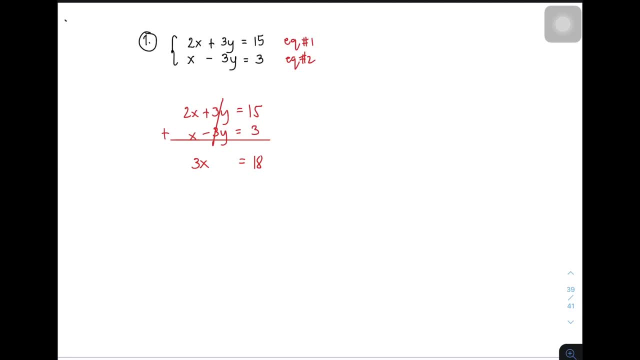 As you can see, we eliminated the variable y and our remaining variable is the variable x. So what this means is we need to solve for the variable x. So solve this: Simply divide it by 3.. Cancel this, It will become 1.. So your x is equal to 6.. This is the first value of your variable. 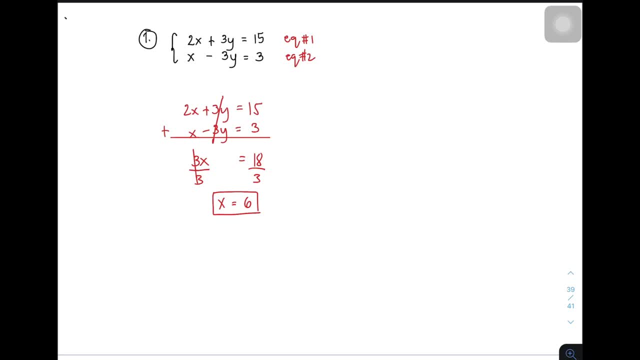 which is x. Since we got the variable x, we need to solve now for y. Solve for y, Because y is the only remaining variable. So, sir, how do we solve y? You can use between the first equation or the second equation. 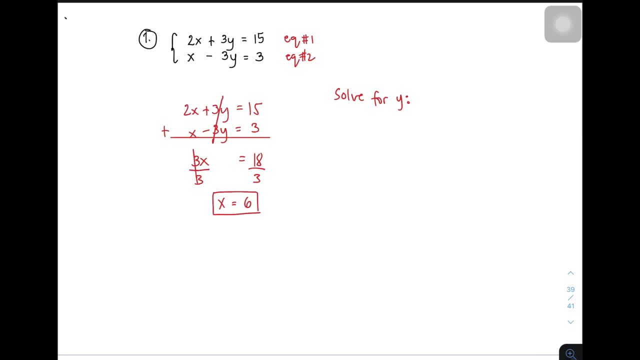 For me, I will be using…. Let's try the first equation. So you have: 2x plus 3y is equal to 15.. Sir, Sir, can we also use the second equation? Yes, you can, As long as your x is equal to 6.. 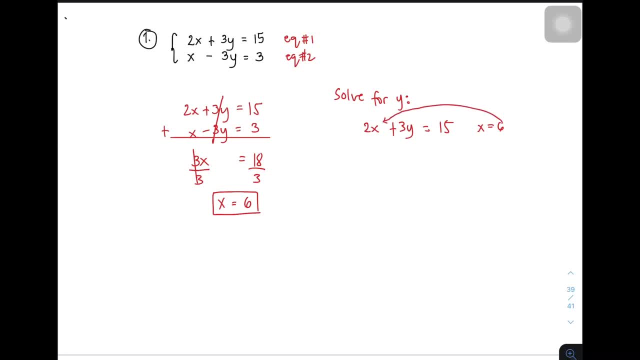 Let's plug in our 6 to the variable x, So you can have this equation: 2 times 6 plus 3y is equal to 15.. Simplifying this equation, this is 12.. 2 times 6.. 12 plus 3y is equal to 15.. 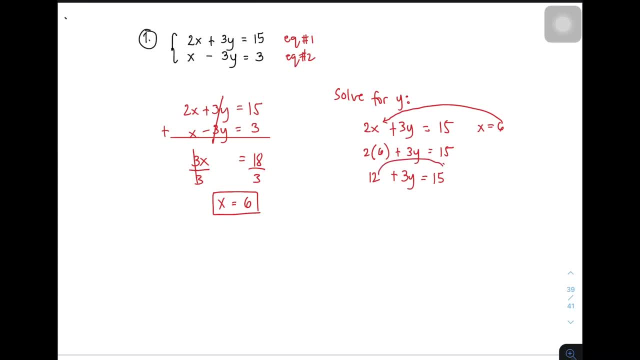 And then our target is to solve for y. Let's transpose this number on the other side. So your new equation is: 3y is equal to 15 minus 12.. Simplifying this one, this will give you 3y is equal to 3.. 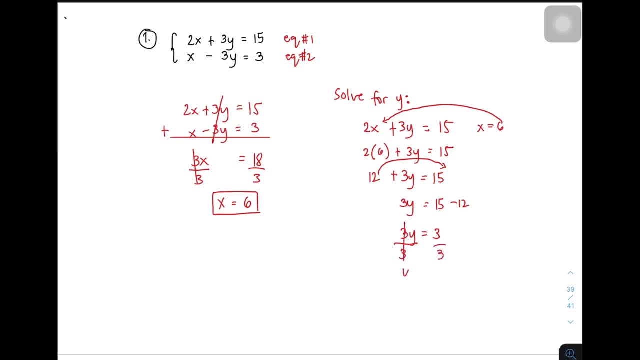 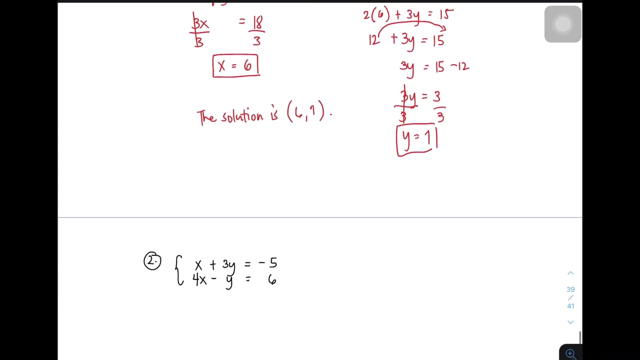 To solve for y, divide it by 3.. So your y is equal to 1.. This means that the solution is 6 comma 1.. This is the correct answer for item number 1 for the given system. Now let's move on with item number 2.. 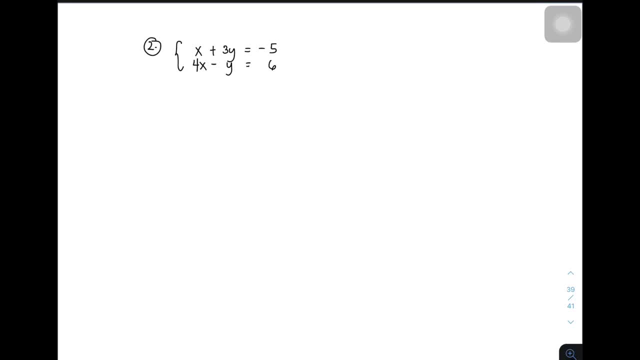 Now we have the given system: x plus 3y is equal to negative 5.. This will serve as your equation number 1.. And 4x minus y is equal to 6.. This will serve as your equation number 2.. 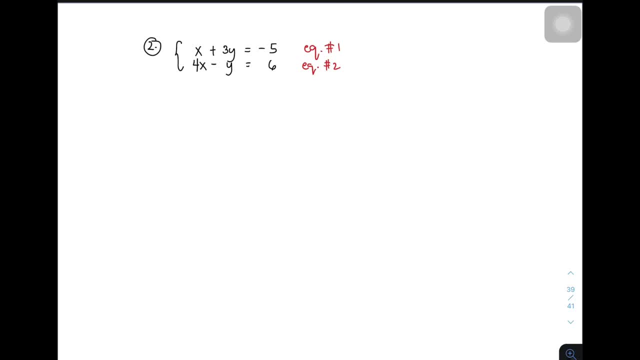 So I told you earlier, we need to eliminate a variable for us to find the value of the other variable. So, sir, how do we do that? You will find a variable with the same coefficient but with different sign. But in our given system, number 2,. 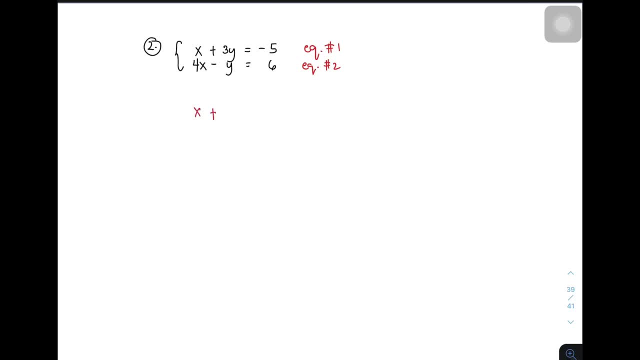 we don't have that kind of case. So you have: x plus 3y is equal to negative 5. So your one is: 4x minus y is equal to 6. So, sir, does that mean that we can't eliminate it? 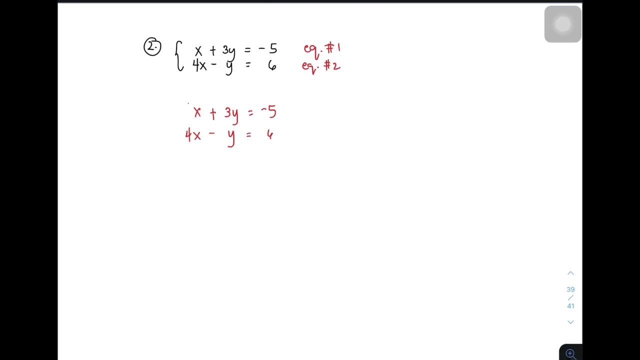 No, We will find a way. We will be multiplying the first equation by negative 4.. Sir, why do we need to multiply by negative 4?? This is the simple reason. When you multiply negative 4 by x, it will become negative 4.. 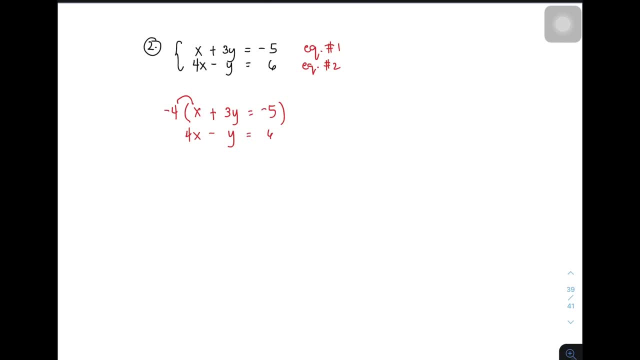 So when you add negative 4x plus 4x, it will become 0. That is its purpose. So you have negative 4x. What will it become? Let's just multiply Negative 4x And then this negative 4 times 3y. 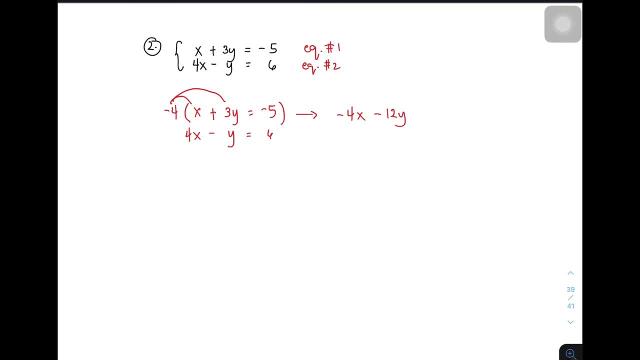 It will become negative 12y. Again, let's multiply by negative 4.. It's equal to 20, because it's negative. And then copy your second equation. Just copy it. You have 4x Minus y is equal to 6.. 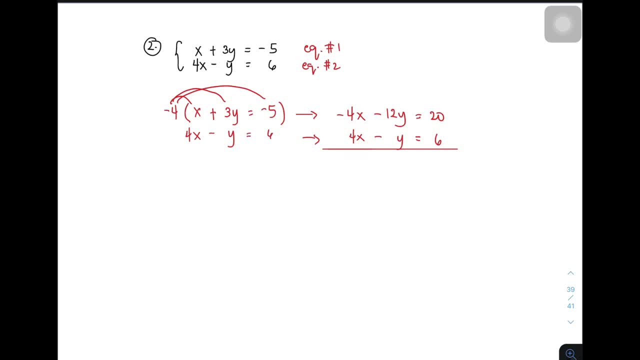 So, as you can see, we can eliminate this part, because negative 4x plus 4x is 0. It will be cancelled or become 0, in other words, And then adding negative 12y and negative y, This will give you negative 13y. 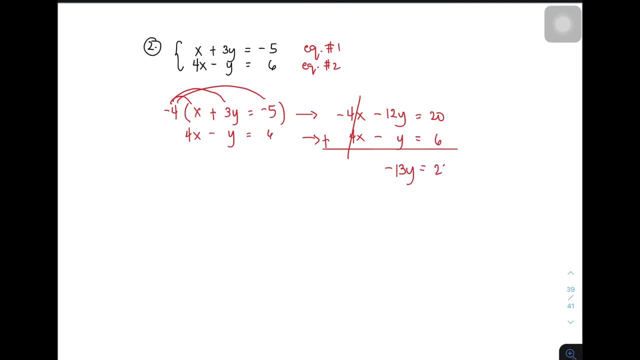 And this part it will give you 26.. Dividing both sides: Dividing both sides of the equation by negative 13.. It will give you: y is equal to negative 2.. This is the value of y. Now, since you already have the value of y, which is negative 2, we can now solve for x. 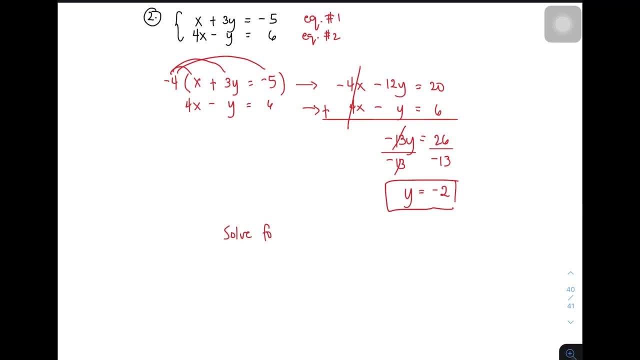 Let's solve for x. Solve for x For the variable x. what I will do is the equation number 1.. I will be using equation number 1.. x plus 3y is equal to negative 5.. Remember, your y is equal to negative 2.. 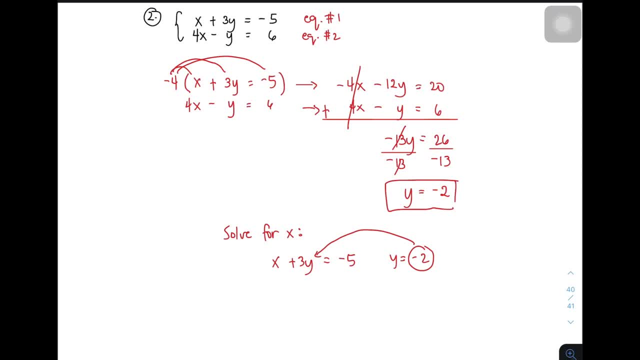 We will replace this negative 2 with the variable y. Okay, So you have x plus 3 times negative, 2 is equal to negative 5.. Let's simplify this: x minus 6, because 3 times negative, 2 is negative, 6 is equal to negative 5.. 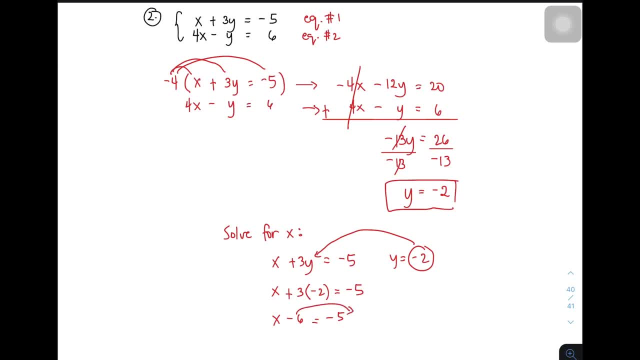 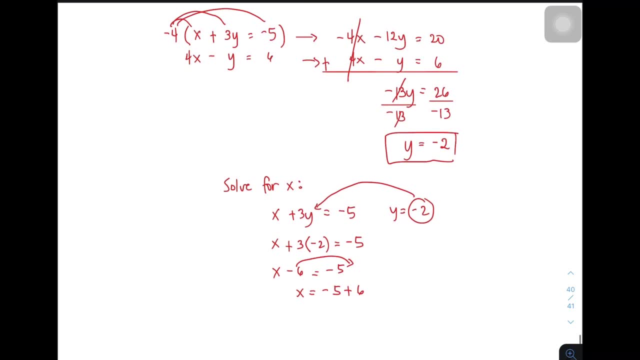 Let's transpose the negative 6 on the other side of the equation. This will give you: x is equal to negative 5 plus 6.. Meaning, if we simplify this, that is, x is equal to 1.. This is the value of x. 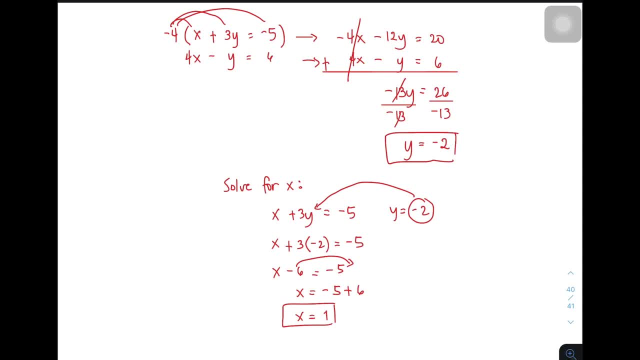 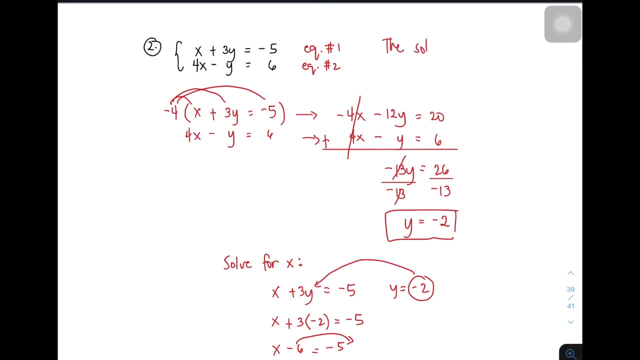 Now, what does this mean? Now, what does this mean if your x is equal to 1 and your y is equal to negative 2?? It means the solution is 1 comma negative 2.. That's it, For example number 2.. 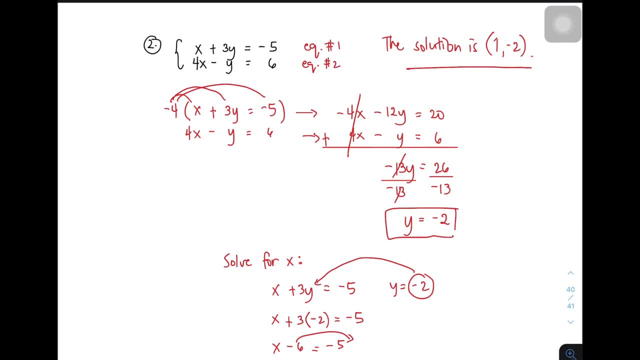 This is our answer, Okay, So if you have a question about the solution that we have, you can comment down below in our video. Again, if you are new to my YouTube channel, don't forget to like, subscribe and hit the bell button to be updated on our future uploads. 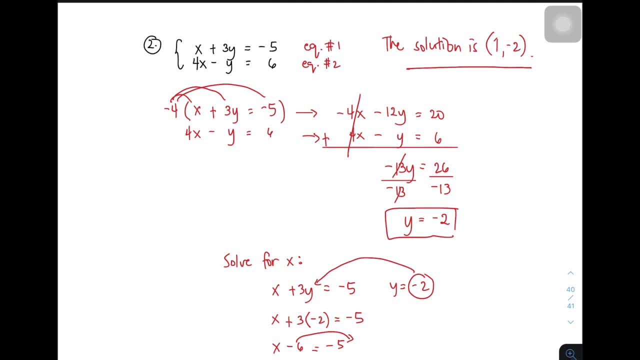 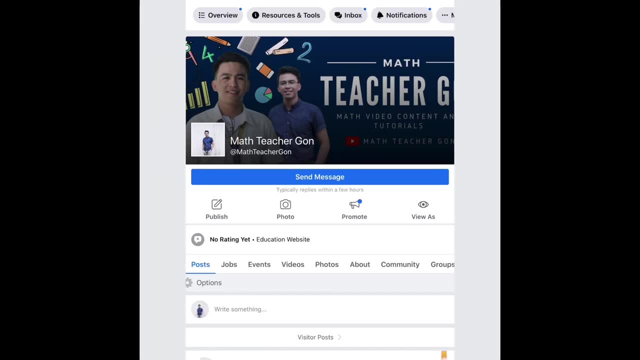 Again, I am Teacher Gon. Thank you very much. Bye-bye, Hi guys. You can also like and follow our Facebook page, which is named as Math Teacher Gon. We are uploading this for our followers on Facebook, So I hope that you will also follow it. 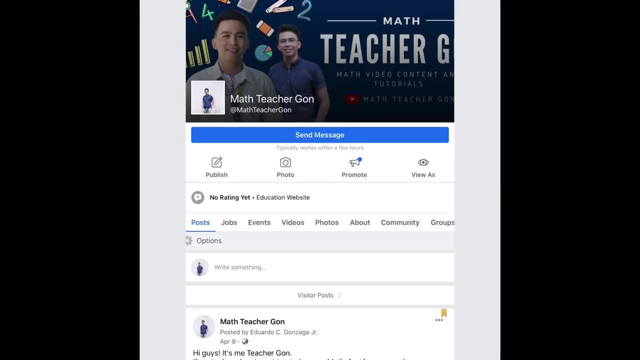 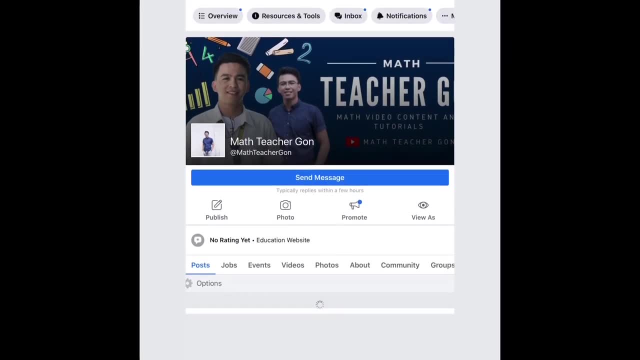 And you will see it, Or you can visit our page. So right now we have 14,000 followers and likers of this page And I hope that we can join you on this page. God bless.